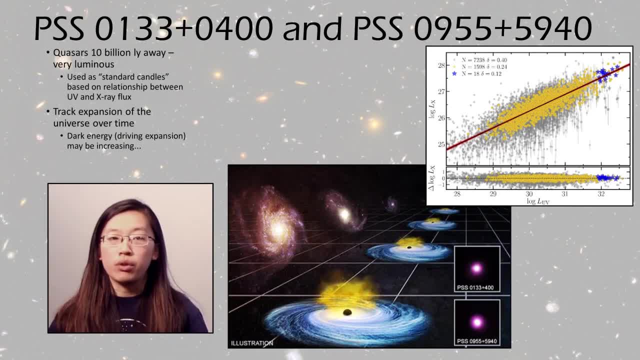 Next we have PSS 0133 and 0955.. So these are two quasars about 10 billion light-years away. As you know, quasars are very, very bright, and so they can be seen from very, very far distances. 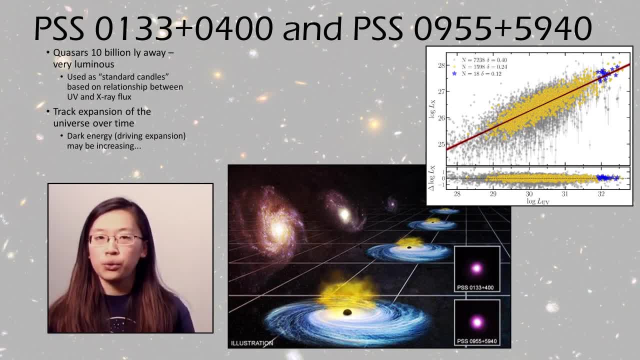 And you know, wouldn't it be great if you could use these as standard candles? And it turns out you can. There's a relationship between the UV and the X-ray flux of these quasars, and from that we can determine their distances. 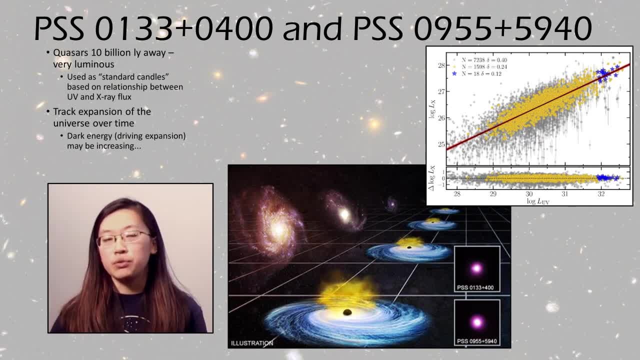 And using their distances, we can track the expansion of the universe over time, since we know their distance and we know how far ago it was, And based on these quasars, it appears that dark energy which is driving the expansion of the universe. 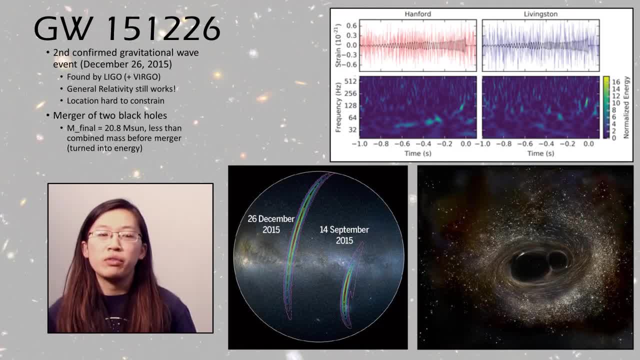 might be increasing over time. Lastly, we have a couple of DSOs that are related to gravitational waves, So GW 151226 was the second confirmed gravitational wave event found in December of 2015.. So this was, of course, a sensitive gravitational wave event. 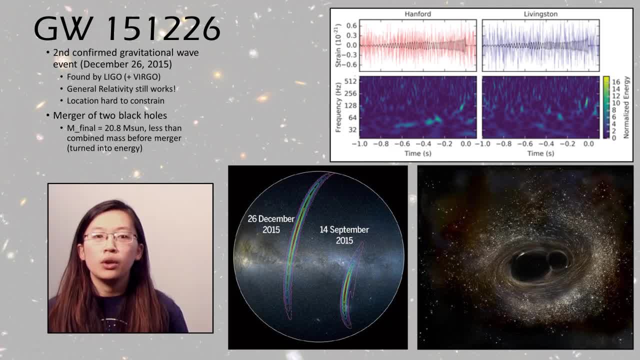 It was discovered by LIGO and also Virgo. So what we were able to tell from this event is that general relativity does indeed still work, because it confirmed a lot of what we expected based on general relativity. However, this was kind of a hard event to follow up. 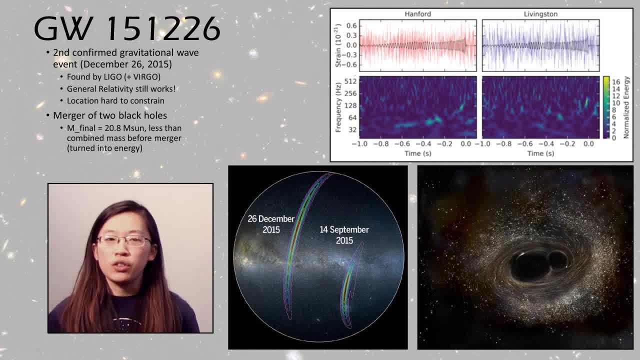 because, as you can see in the bottom left there, its location on the sky was kind of hard to constrain. So this is thought to have come from a merger of two black holes With a total mass of a total final mass of 20.8 solar masses. 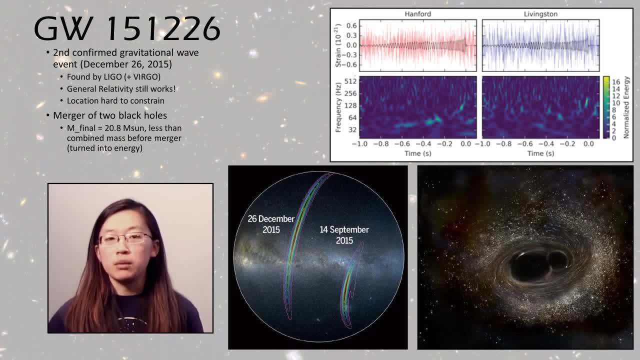 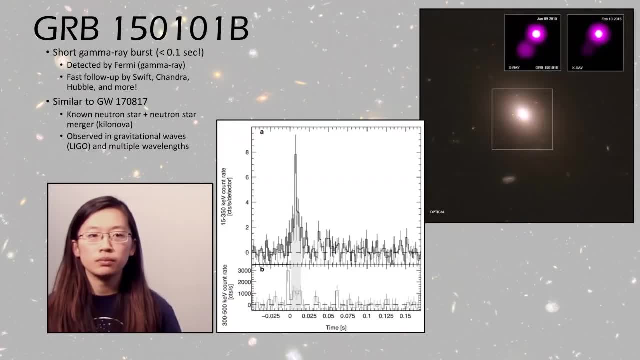 So this is actually less than the calculated mass of the two black holes before the merger, because some of that mass was turned into energy that we then saw. Lastly, we have GRB 150101B, So this was a gamma ray burst, GRB. 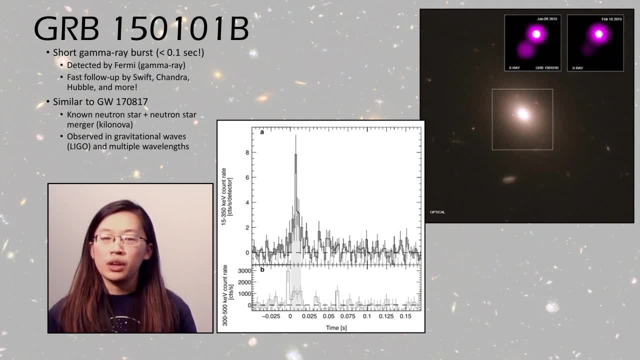 This was a short burst, which is less than 0.1 second, that was detected by the gamma ray satellite Fermi, And then it was quickly followed up by Swift, Chandra, Hubble and many more observatories. So this DSO is special because it was similar to a known neutron star plus neutron star merger. 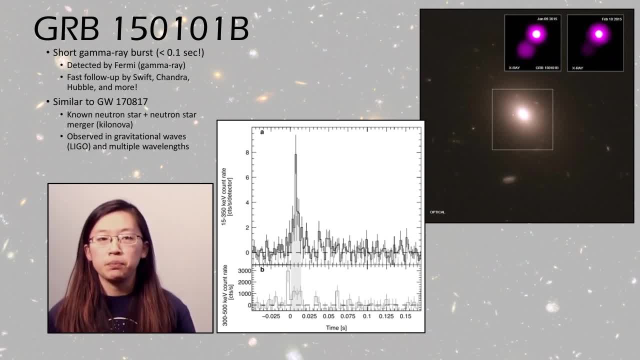 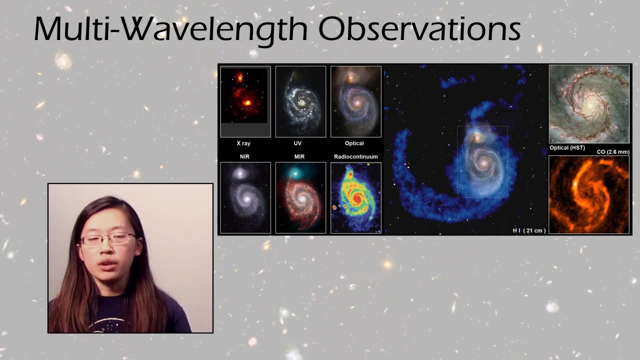 which was called GW170817.. And so it's thought that, because this one and that one were so similar that they actually are the same type of event, even though we couldn't observe the gravitational wave for this event, Now that we've gone through the DSOs. 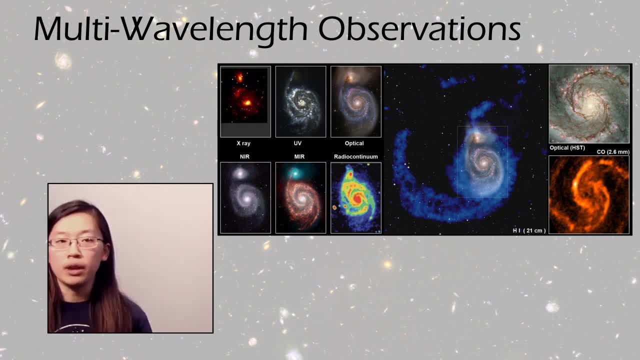 I want to go over a few more things that you might find helpful as you prepare for the astronomy event. One of these is using multi-wavelength observations. As you can see, this galaxy looks very, very different in the X-ray as opposed to the optical as opposed to the infrared. 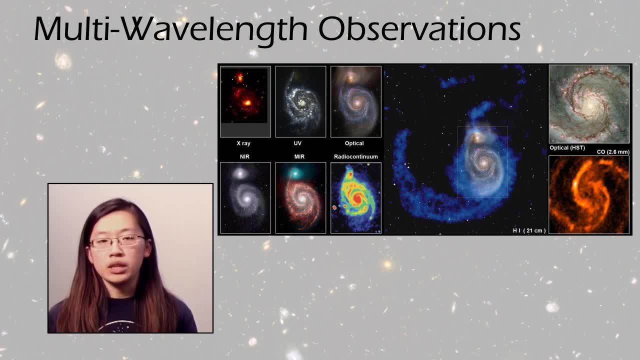 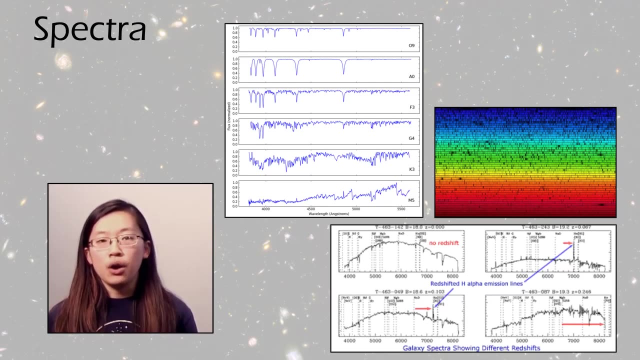 So all these different wavelengths serve to highlight different parts of this galaxy and the different processes going on there. So this is why it's important to take a look at many of these DSOs in multiple wavelengths We also have spectra which tell us a lot about the chemical composition of our DSOs. 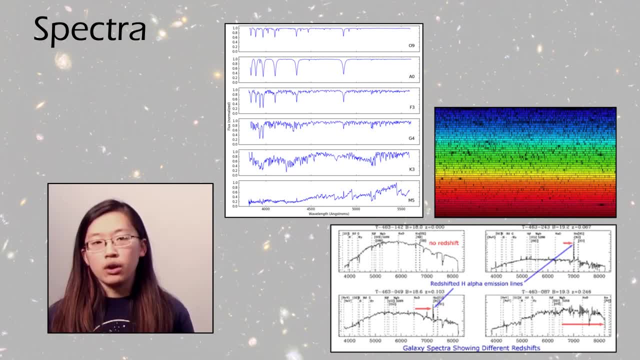 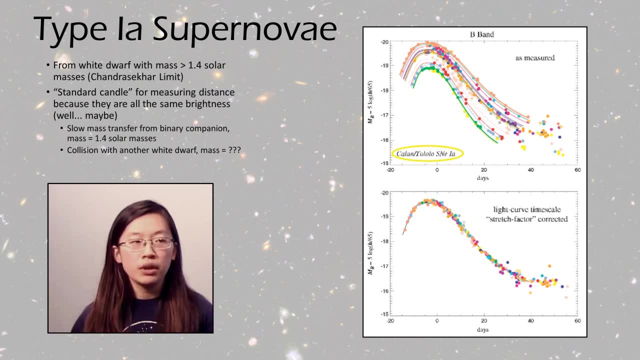 as well as something about how they emit energy, whether they're absorbing or emitting in these elements. Moving on to a couple of topics that are relevant, A Type Ia supernovae: These come from white dwarfs with masses greater than the Chandra-Sacar limit. 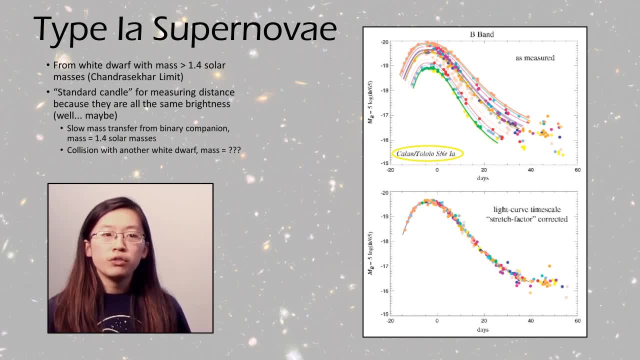 which is about 1.4 solar masses, And these are often used as standard candles for measuring distances because they ought to all be the same brightness. However, we're finding that this is not necessarily true. Classically, we thought that a lot of these Type Ia supernovae. 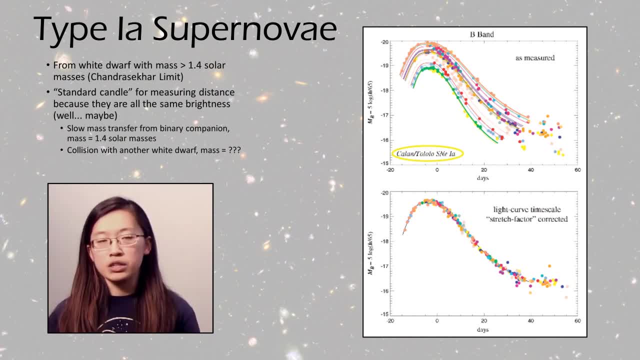 came from a white dwarf that was slowly, slowly gaining mass from a companion And therefore, when it blew up, its mass would be pretty close to 1.4 solar masses. However, we're discovering that a significant fraction of these supernovae 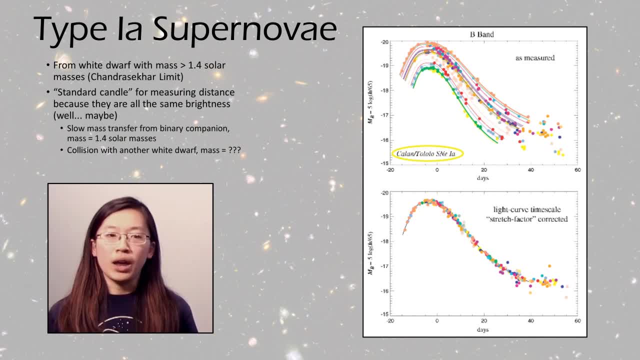 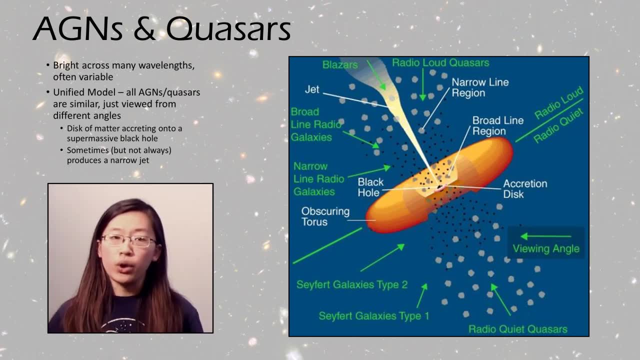 actually come from the collision of two white dwarfs, which means we don't actually know the mass before it went supernova. Next we have AGNs and quasars. Like I said earlier, these are often defined by being bright across many wavelengths. 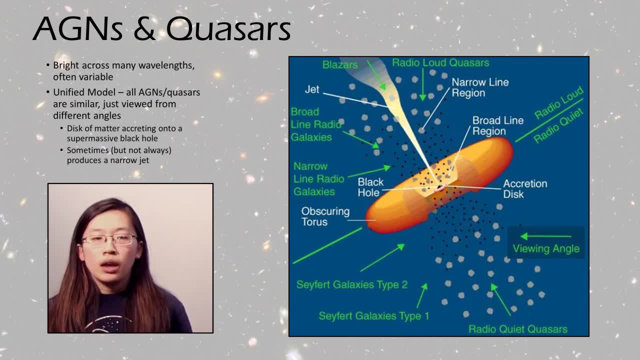 and being variable brightnesses, And there's a unified model of AGNs which says that they're all pretty much the same thing. It's a supermassive black hole with a disk of matter around it, and sometimes it produces a jet. 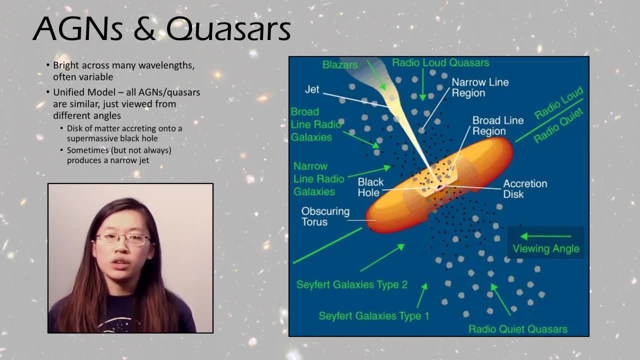 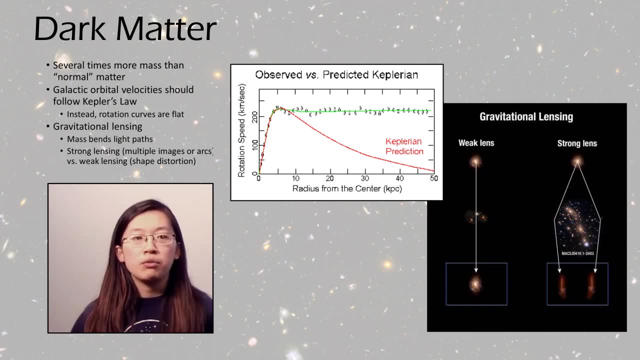 And all the different kinds of AGNs and quasars that we see are just from viewing this system from different angles. Another big topic for this year is dark matter, which makes up actually a lot more of the universe than normal matter. So dark matter was discovered by Vera Rubin. 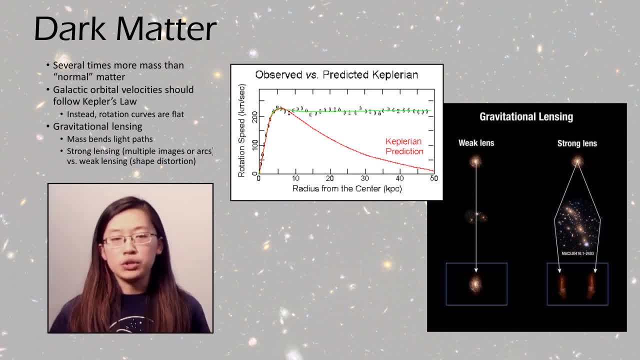 when she found that, instead of following Kepler's law, the orbital velocities of stars around the center of the galaxy actually stayed pretty flat, which meant that there must be some kind of invisible mass causing this. Another important thing about dark matter is that it causes gravitational lensing. 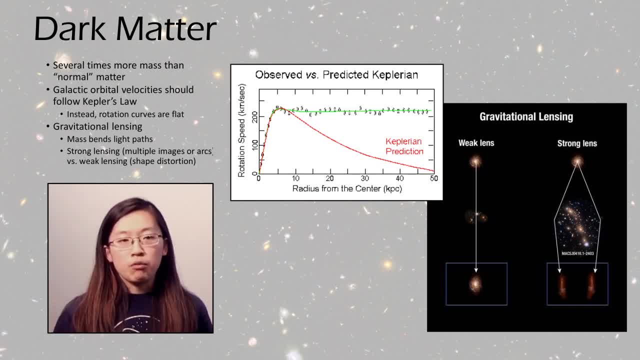 So, based on relativity, a lot of mass will bend the path of light, And gravitational lensing is when we have more light from a distant object being bent by the mass of a closer object, And there's different kinds of lensing. 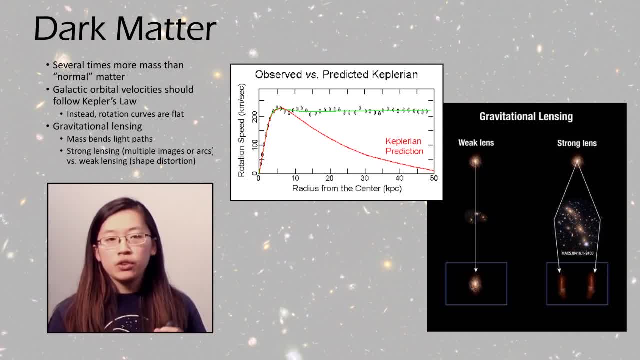 Such as strong lensing, which is where you see multiple images or you see those very, very distorted arcs, versus weak lensing, which is just a small distortion of the shape- Another big topic for this year that I didn't really touch on earlier. 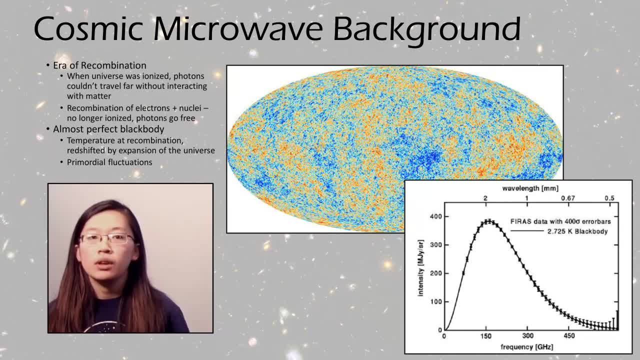 is the cosmic microwave background, or CMB. This comes from the era of recombination, So early in the history of the universe. everything was ionized and the photons couldn't go anywhere without interacting with something. However, when the universe cooled off enough, 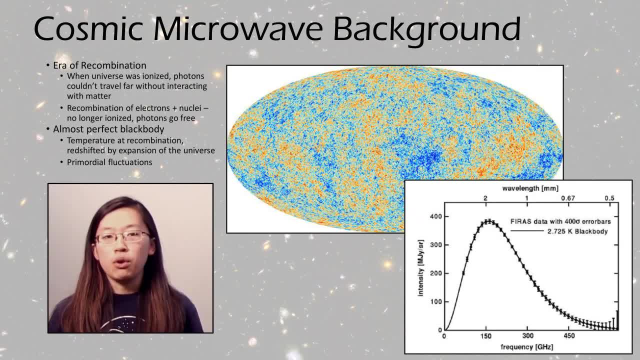 that the electrons managed to recombine with their nuclei to form atoms. the universe was then no longer ionized, and the photons could go on their merry way, And so the cosmic microwave background is the photons that we see from this time, but redshifted by the expansion of the universe. 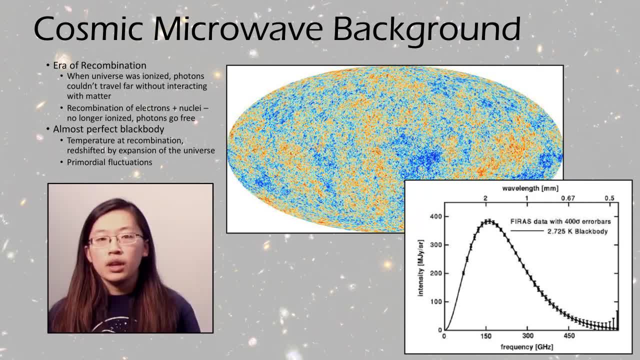 And in fact the CMB is almost a perfect block body, except, as you can see in that top image. there there are some very, very small fluctuations and this is just caused by the randomness of the early universe. But those fluctuations are very important for driving the later structure of the universe. 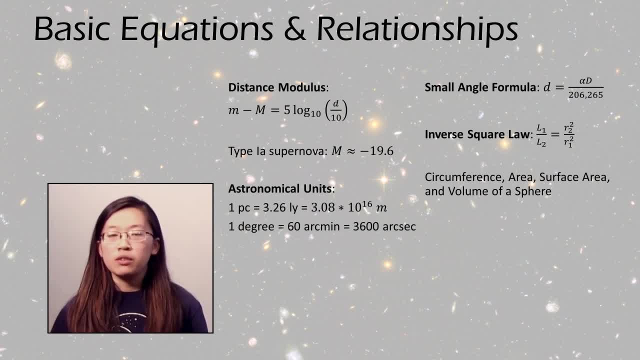 I know that was a bit of a whirlwind tour of those topics, but I think that it's important that, especially if this is your first time doing astronomy or the first time that you're dealing with galaxies, it's important that you be exposed to these concepts and ideas. 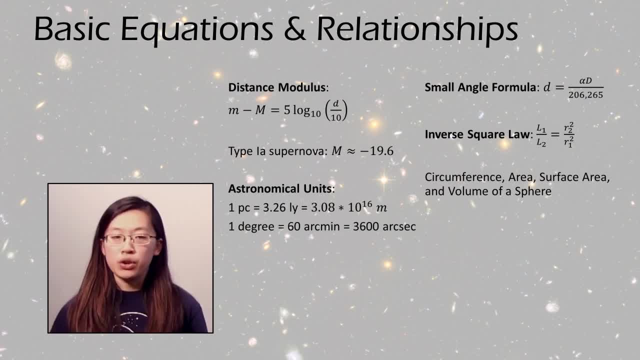 so that, even if you don't fully understand them right now, later when you hear them again, you'll look back and be like: wait, I heard about that. So, moving on to some of the basic math that you'll be required to know for astronomy, 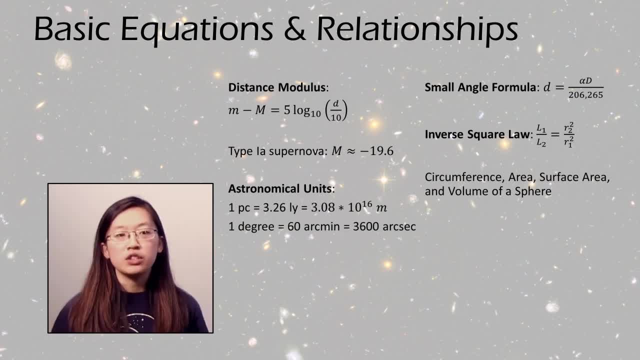 here are a couple of the basic equations. There's the distance modulus, which lets you determine the distance of an object based on its apparent and absolute magnitudes, or rather how bright it appears to be and how bright it's known to be. 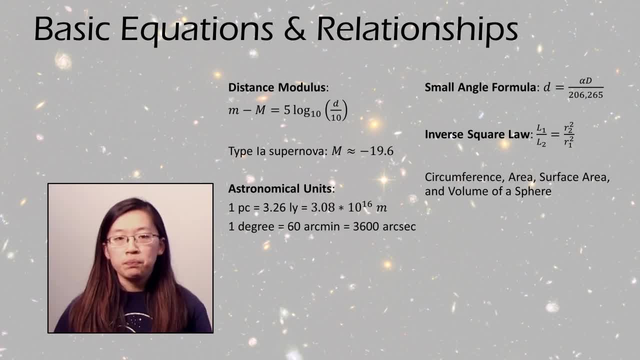 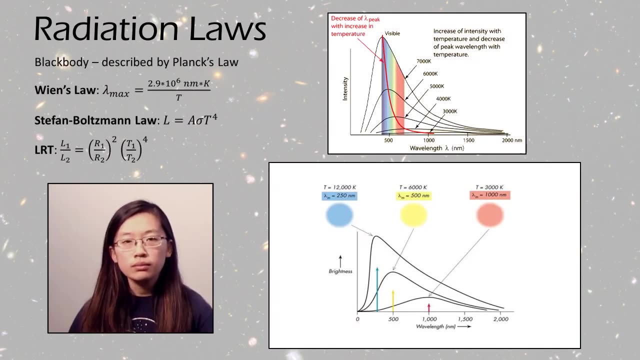 There's also the small angle formula and the inverse square law, as well as just knowing some things about the weird units that are used in astronomy, as well as things like basic geometry, the circumference area, volume of a sphere, things like that. 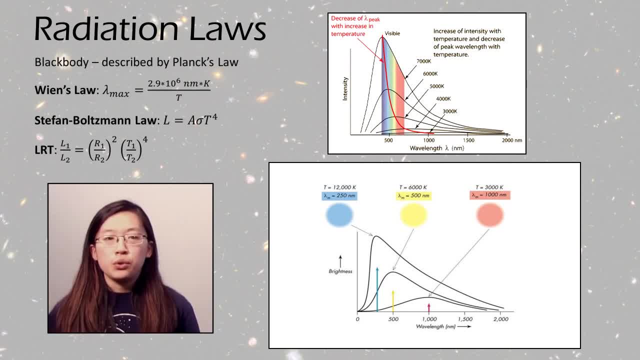 Our next topic would be radiation laws. So many objects in space radiate as black bodies, so these are described by something called Planck's law and, based on this, there's Wien's law, which lets you find the wavelength at which the maximum amount of light is emitted. 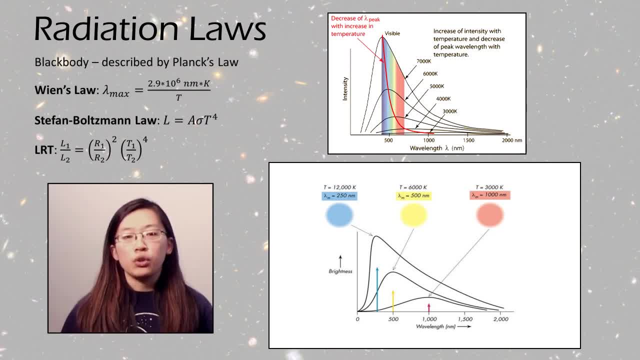 and the Stefan-Waltzmann law, which lets you find the total amount of light that's emitted over all wavelengths, And for stars there's often a very handy relationship between the total luminosity and the radius and the temperature, which is called LRT. 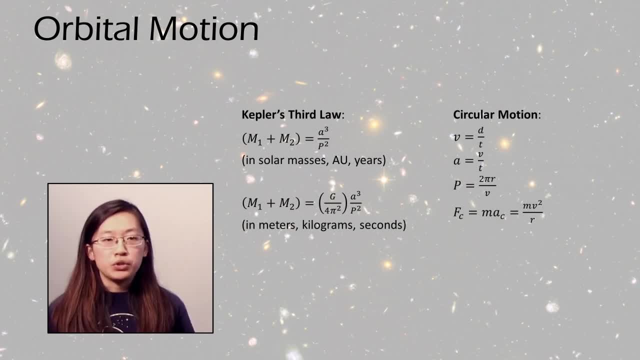 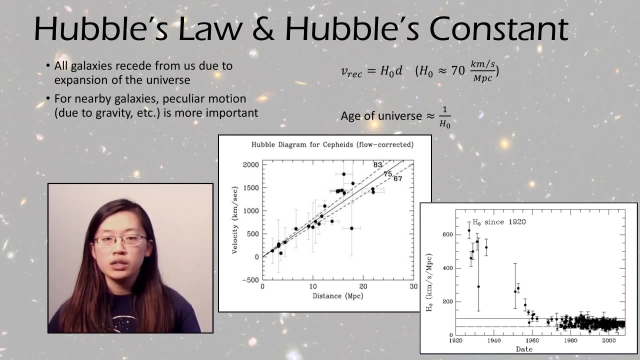 Next we have orbital motion. There's Kepler's third law and there's also a bunch of equations that you may or may not be familiar with from physics that describe circular motion. Last, on the math topic, there's Hubble's law and Hubble's constant. 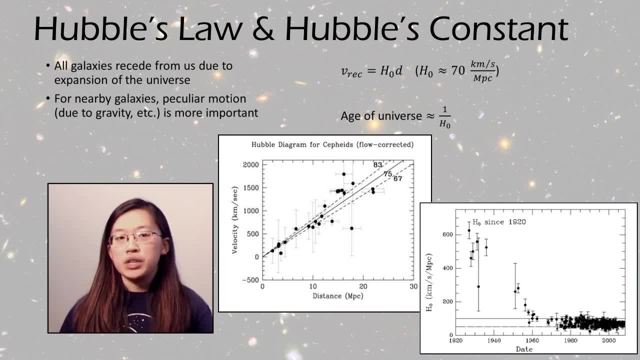 So all galaxies are receding from us due to the expansion of the universe. For nearby galaxies, often this is overpowered by peculiar motion. such as the Milky Way and Andromeda are moving towards each other due to their mutual gravity, But as we go out into further galaxies, 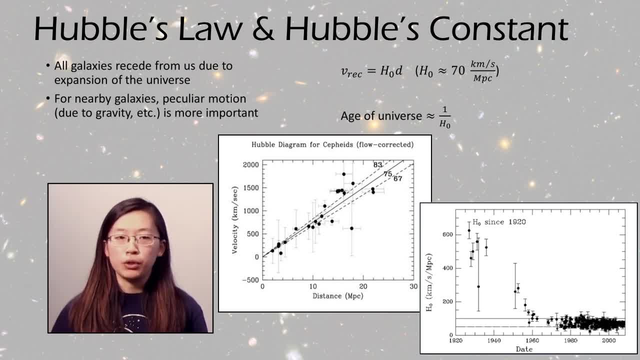 they will generally be moving away from us due to the Hubble flow. So Kepler's law and Hubble's law basically says that you know this distance is proportional to some constant times: that recessional velocity And the value of Hubble's constant. 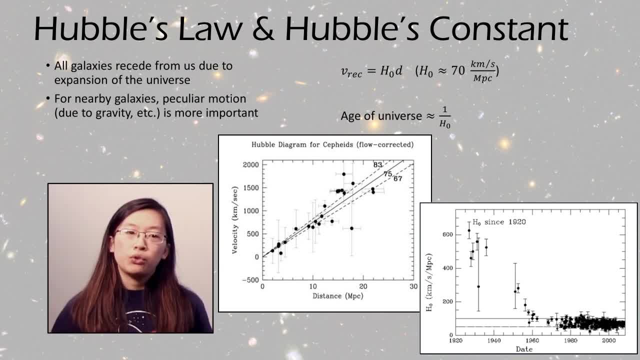 is generally about 70 kilometers per second per megaparsec, So you might notice that this is actually a unit of one over time, since the kilometers in the megaparsecs can cancel out, And thus the age of the universe. 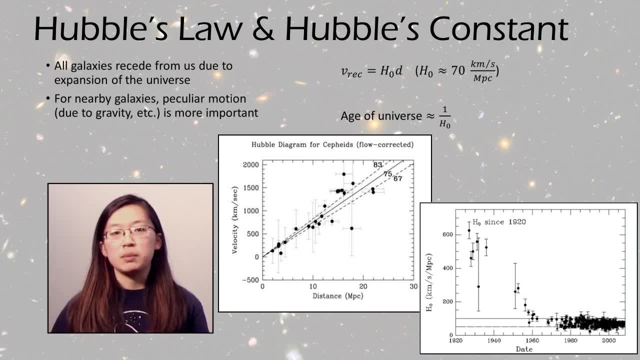 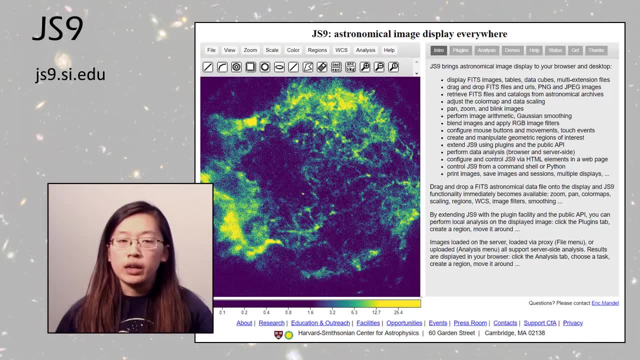 is roughly given by the Hubble constant, since Hubble's constant describes the expansion rate. Next, I would like to mention JS9, which is an important part of this event. JS9 is based on DS9,, which is used for looking at. 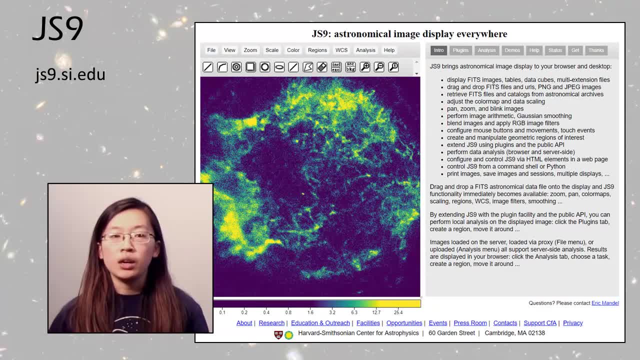 and also analyzing astronomical images and data. JS9 can be found on the internet at js9.siedu, complete with a tutorial on how to use it. So JS9 will be used at nationals this coming year and may be used at regional and state competitions as well. 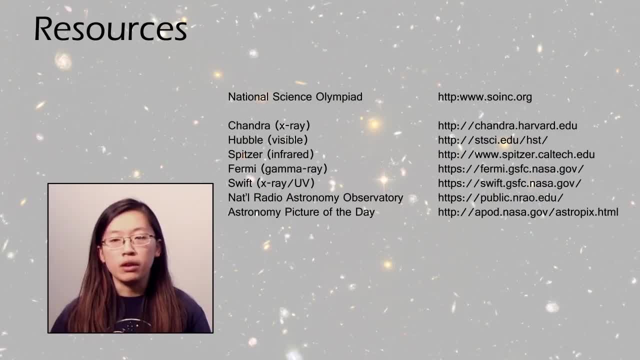 Here are some resources that you might find useful as you prepare for the astronomy event. Of course, there's a lot of stuff at National Science Olympiad at soincorg and also a lot of good stuff at the websites for all these NASA missions. 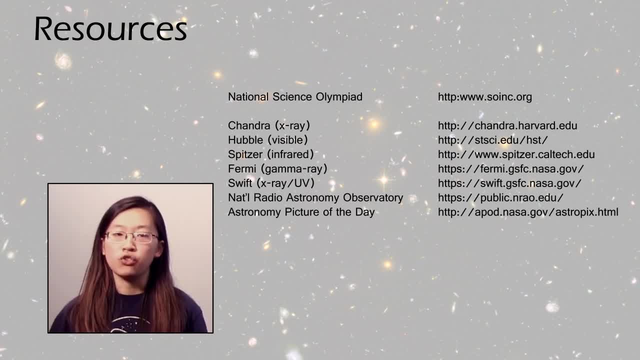 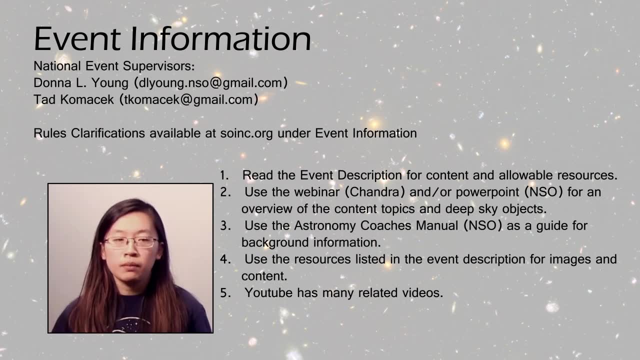 as well as the National Radio Astronomy Observatory and Astronomy Picture of the Day, or APOD. Finally, to close out, here's some important information about the event. The national event supervisors are Donna Young and Tad Komacek. Rules and clarifications will be available as usual. 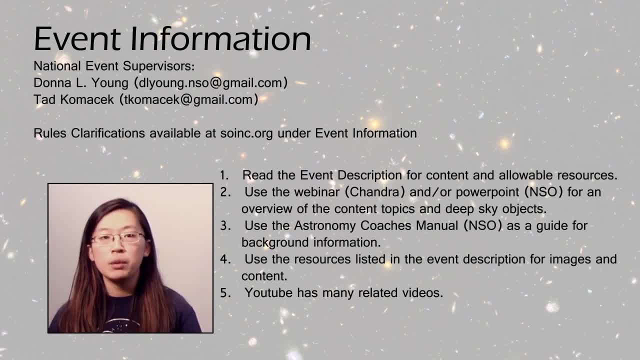 at soincorg under event information. And lastly, just a couple of tips that might help you prepare, Of course, look through the event description, follow the rules. the webinar which you're watching now and the associated PowerPoint are very useful. 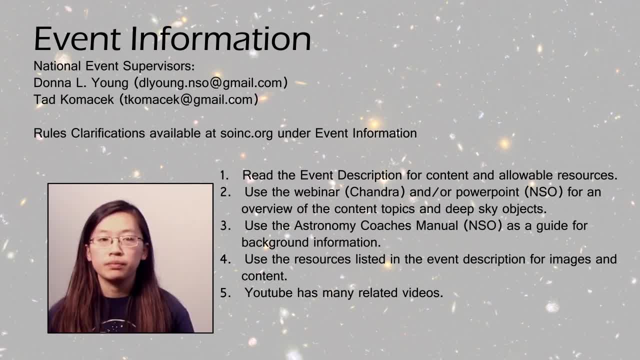 for getting an overview of the topics and DSOs. If you want background information, you can look through the Astronomy Coaches Manual from NSO as well As well. there are many resources that I just listed and they are also listed in the event description. 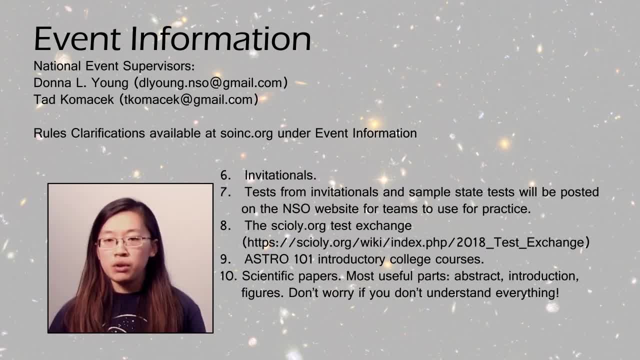 YouTube has related videos. If your team is lucky enough to go to Invitationals, those are good experiences. Tests from Invitational and a sample state test will also be posted on the NSO website for you to use for practice. You can also find many tests.